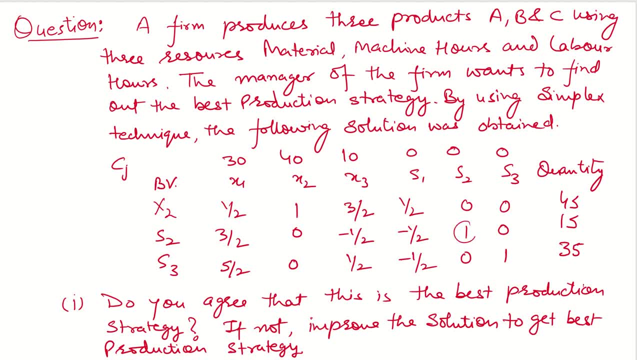 S2, just see: against S2, S2: this is 1 and other are 0. Against S3, S3 is 1 and other are 0.. Now we want to check this by Simplex method. First we prepare the Simplex table using given data. 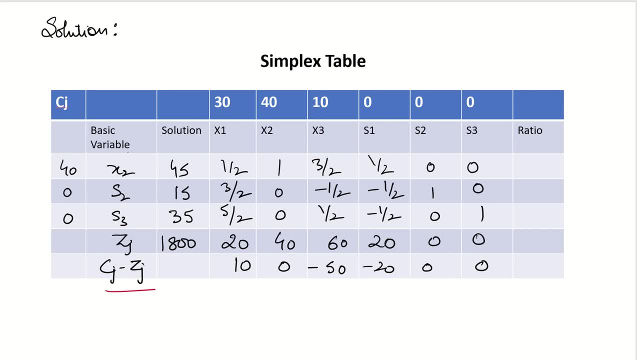 And calculate Cj minus Zj, which is give you net evaluation, And the values in Cj minus Zj are 10, 0, minus 50, minus 20, 0 and 0.. All values are not 0 or negative. 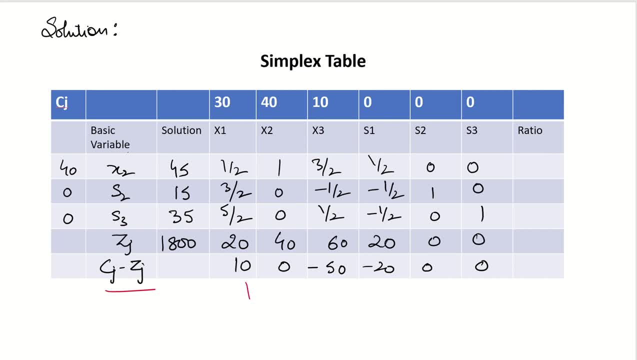 So it is not an optimum solution. Here we will choose 10 as a key column, Which give you X1 as an entry variable. because we will take this as a key column? because 10 is a maximum positive value. Now we calculate ratios. 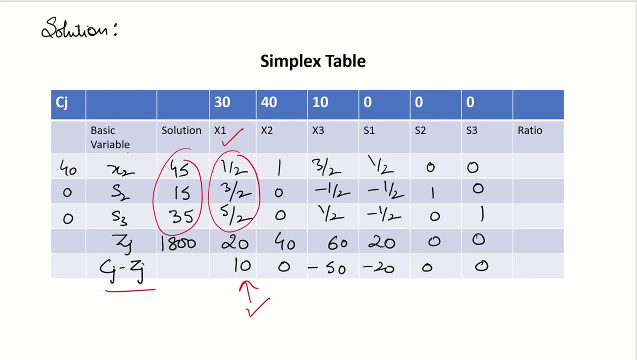 So we will take the solutions, divide by key column elements And we will get the answer 90.. 15 divided by 3, by 2, it is 10.. And this is 14.. And out of this, minimum is 10.. 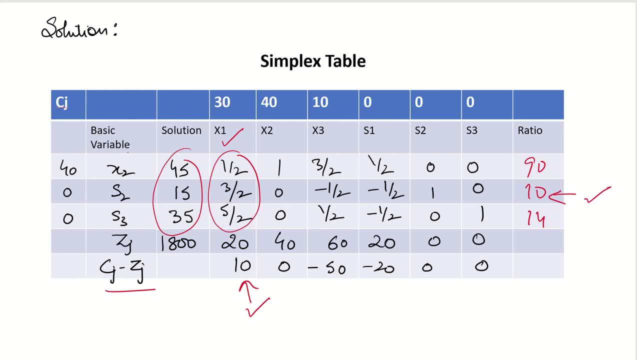 And we will take 10 as a key row And the point of intersection of this key row and a key column give you key element. So 3 by 2 is your key element And this will say this key row says S2 is departing variable and key column says X1 is entering variable. 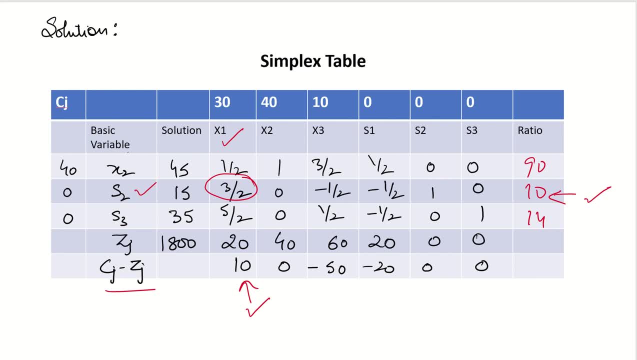 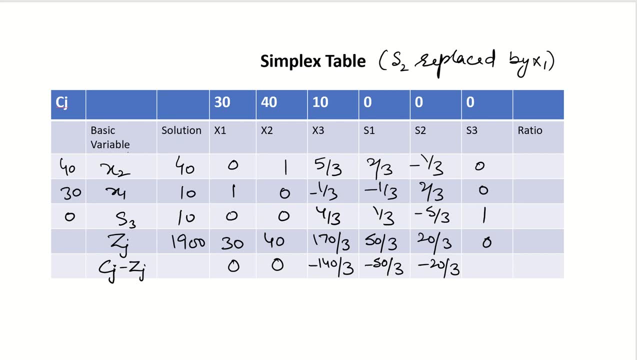 So in the next Simplex table, S2 is replaced by X1.. In the next Simplex table, S2 replaced by X1.. And after making all the calculation, we just see that what is the values in Cj minus Zj, which is net evaluation row. 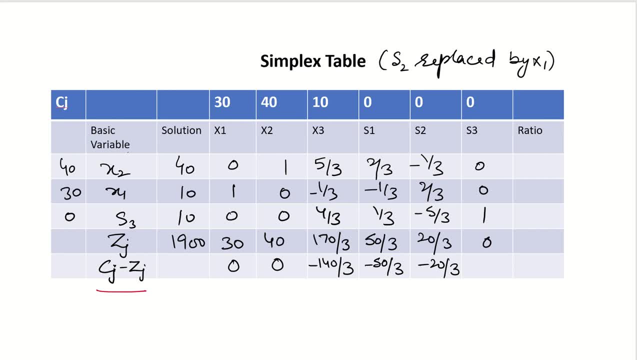 0, 0, minus 1, 40 by 3, minus 50 by 3, minus 20 by 3.. Since all values in Cj minus Zj are 0 or negative, so it is an optimum solution. 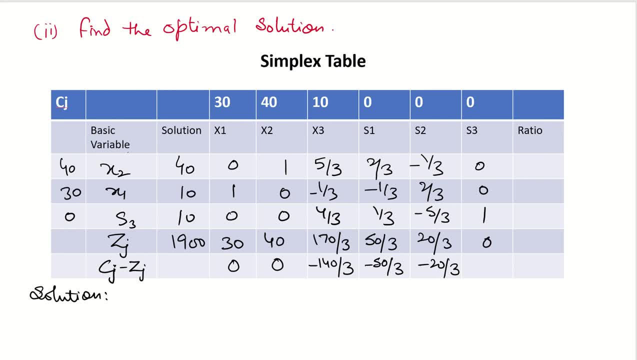 Now in this Simplex table, find the optimum solution. Because all values in Cj minus Zj are 0 or negative, so it is an optimum solution Here. maximum value of Z is 1900 at X1 equals to 10.. 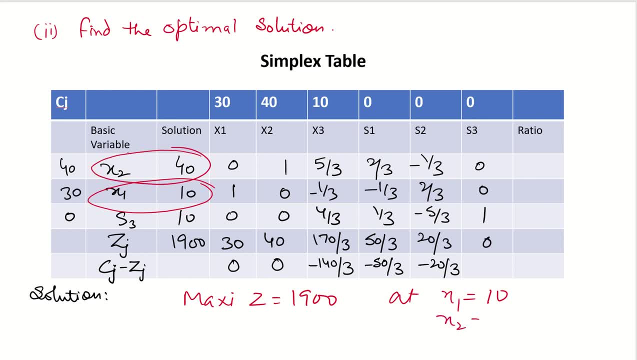 X2 equals to 40.. And X3 equals to 0.. Next question: are all three resources completely used? If not, how much of these resources is unused? Just see in this solution: S1 is 0.. S2 is 0.. 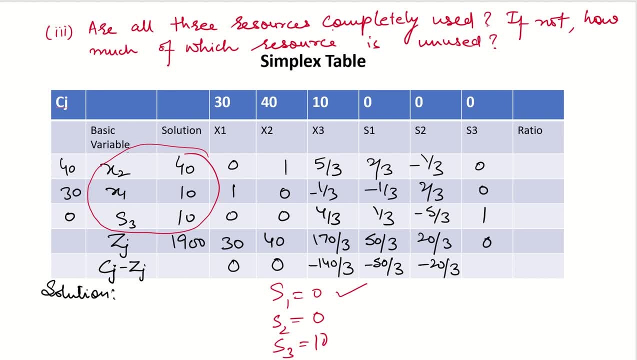 S3 is 10.. This implies first resource is fully utilized, second resource fully utilized and third resource is still available of 10. 10 labor hours. So this resource is underutilized by 10 hours. S1 is material, S2 is machine hours and S3 is labor hours. 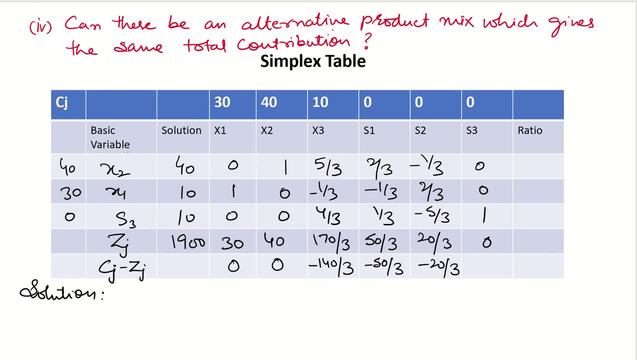 So still 10 hours are available. Next question: can there be an alternative product mix which gives you the same total contribution? Just see that basic variables are X2, X1, and S3.. And X3,, S1, and S2 are known as non-basic variables. 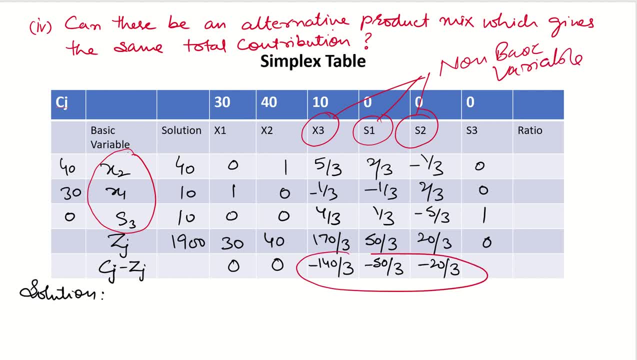 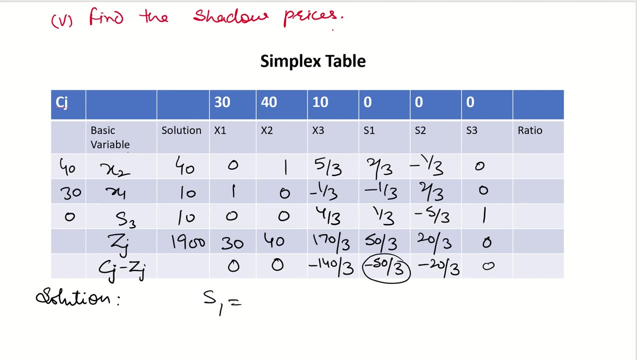 None of the non-basic variables having value 0 in Cj minus Zj. So there is no alternative solution. No alternative solution. Next part: find the shadow prices For S1, shadow prices: 50 by 3 per kg. 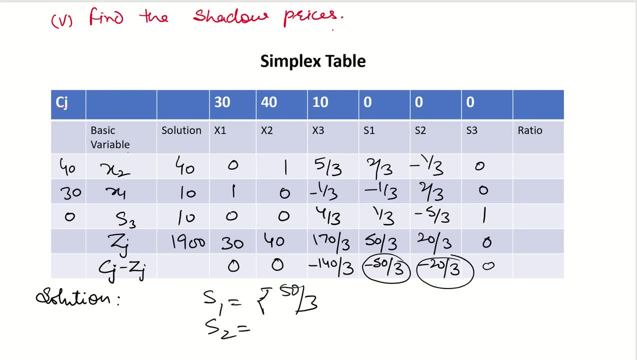 For S2, S2 related to machine hours- 20 by 3 per hour And for S3, S3 related to labor hours, It is 0. Because labor hours are still available- 10. So the shadow price for the labor is 0.. 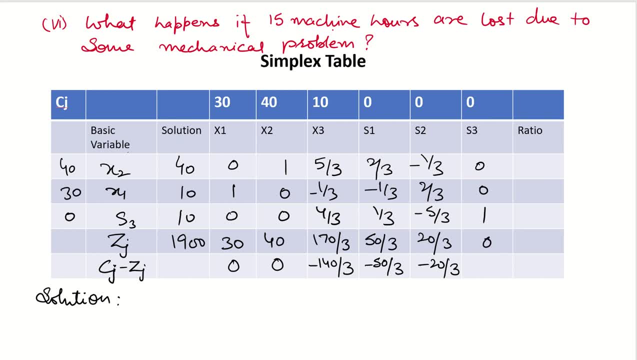 Next part: What happens if machine hours are lost. 15 machine hours are lost due to some mechanical problem. We know that shadow price of the machine hour is minus 20 by 3.. This implies if we lost 1 machine hour there is a loss of 20 by 3 rupees. 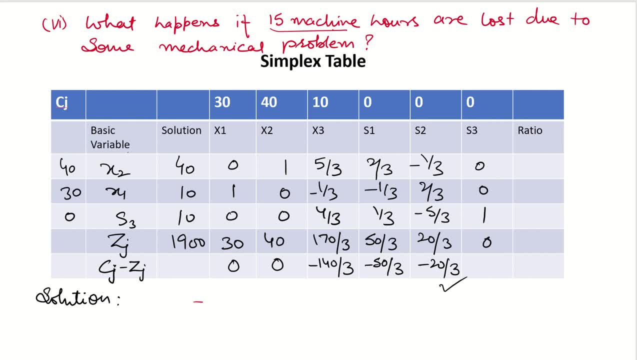 So if we lost 15 hours, so total loss is 20 by 3 into 15.. This implies 100 rupees loss, Loss of rupees 100 in profit And the new profit is 1800.. If there is a loss of 15 machine hours.